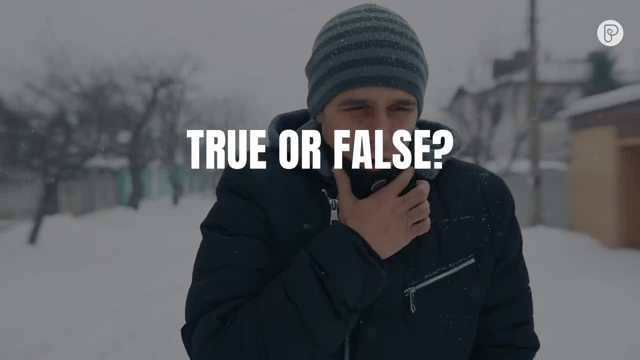 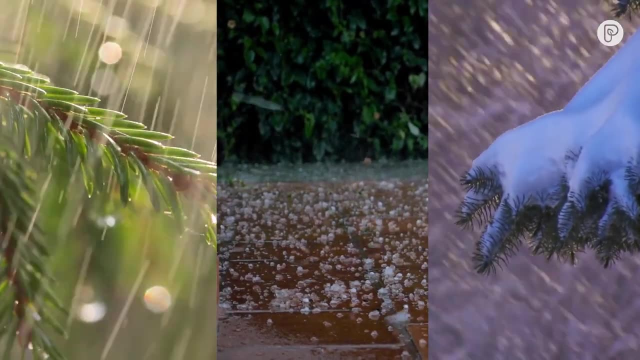 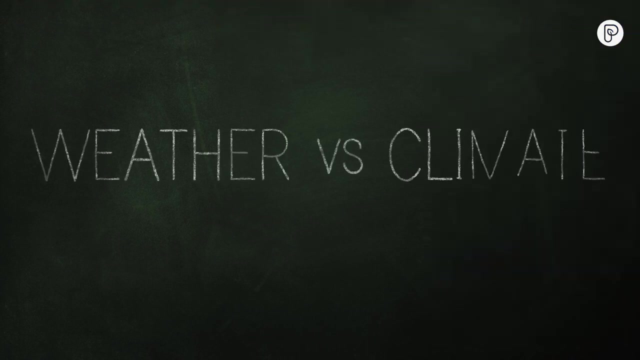 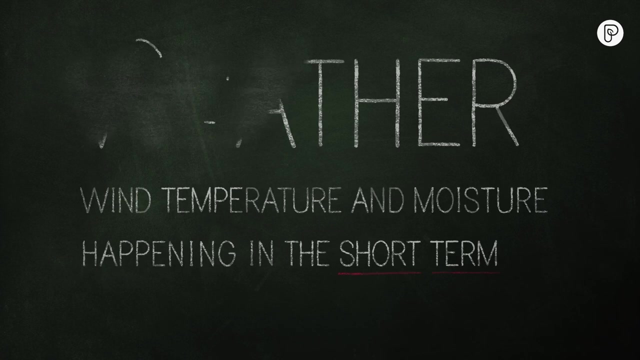 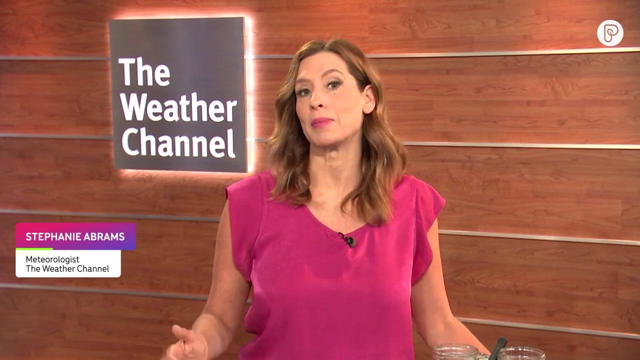 True or false. It's cold outside, so that means climate change isn't real. That's a big false. In many cases, climate change is actually making weather more extreme. Let's separate the facts from fiction. There's a major difference between weather and climate. Weather is the wind, temperature, moisture, those types of things happening right now. in the short term- Think today or tomorrow. Climate is the average of this weather over a long period of time, usually at least three decades, And our planet's climate is changing. 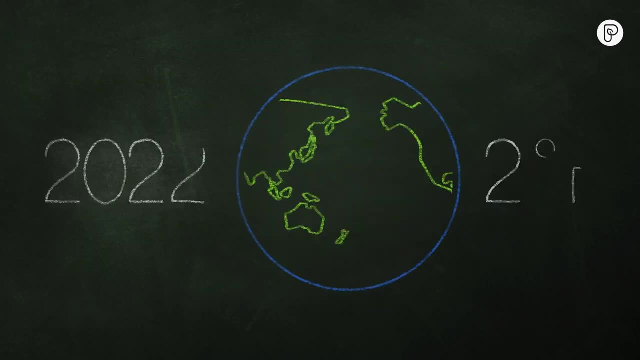 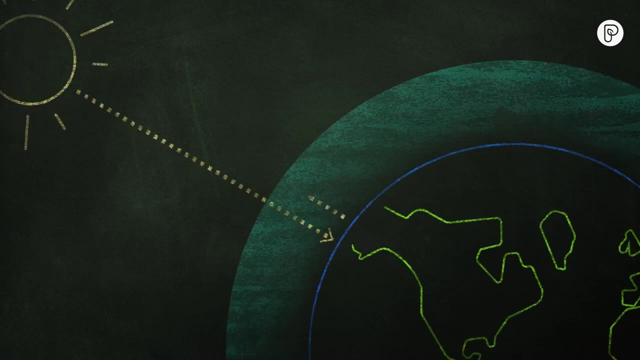 Since 1880, global temperature has increased by roughly two degrees Fahrenheit. One reason for the warming is the greenhouse effect. Sunlight warms the earth and then gets emitted back into the atmosphere where greenhouse gas is released. Sunlight warms the earth and then gets emitted back into the atmosphere where greenhouse gas is released. 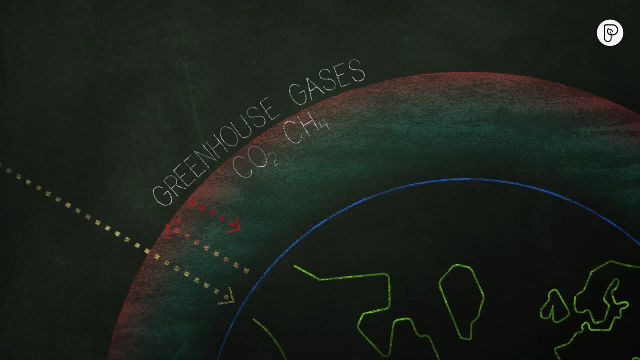 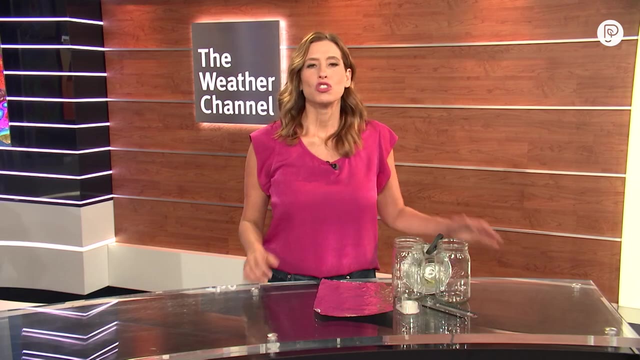 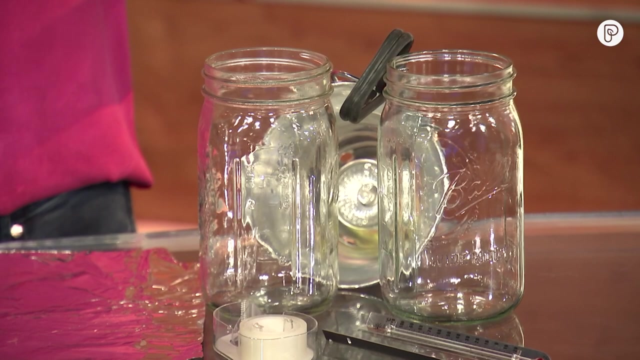 And that's when gases like carbon dioxide and methane absorb and re-radiate some of that heat, warming the planet. But too much greenhouse gas concentration means too much warming. To really visualize this, you can do an experiment in the comfort of your own home. All you need is tinfoil tape, two thermometers, two mason jars and a lamp. 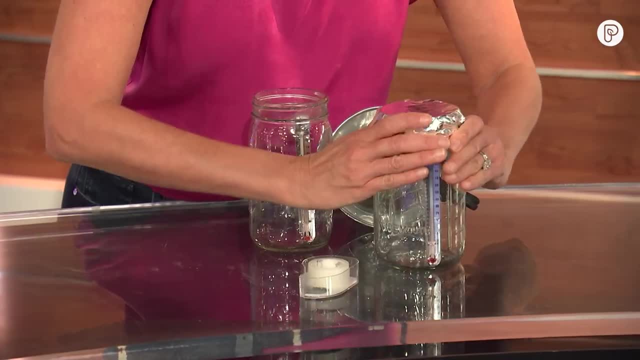